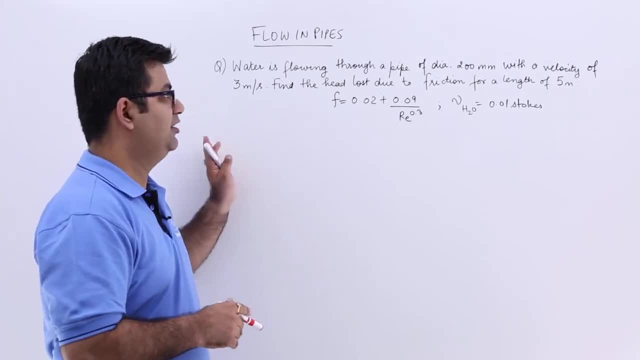 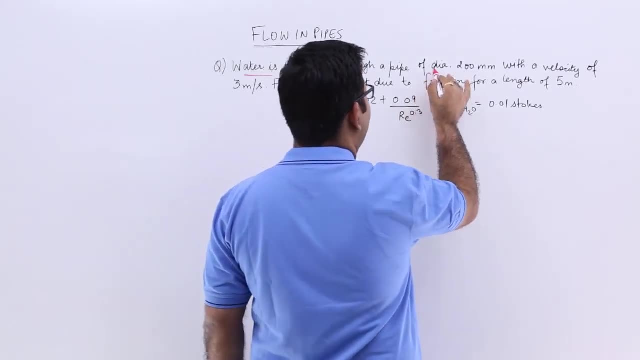 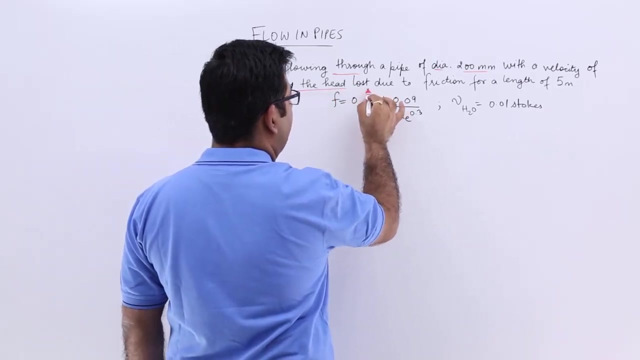 Now let's have a look at a numerical on the friction head losses in pipes. The question says that we have water which is flowing through a pipe of dia 200 mm with a velocity of 3 meters per second. Find the head loss due to friction for a length of 5 meters when. 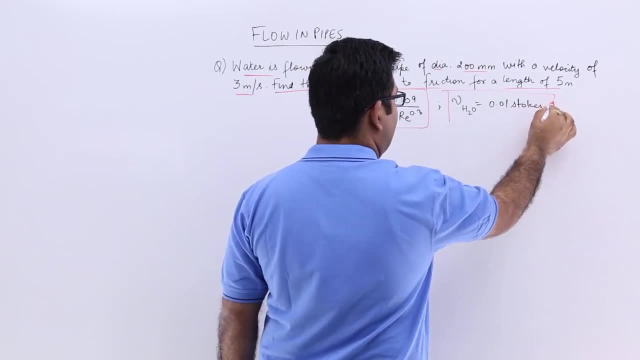 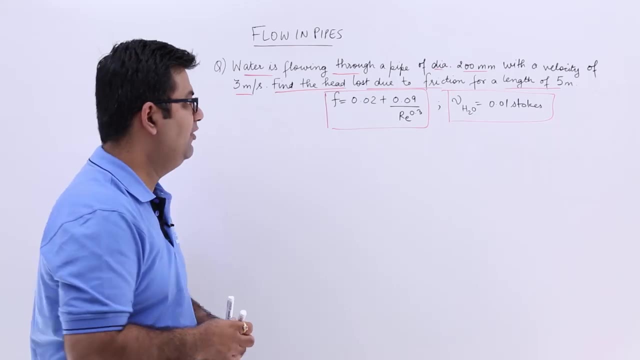 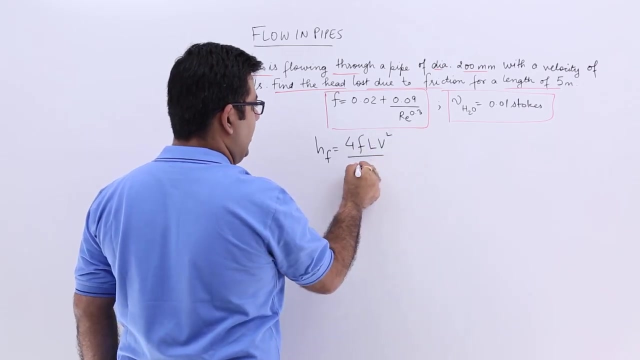 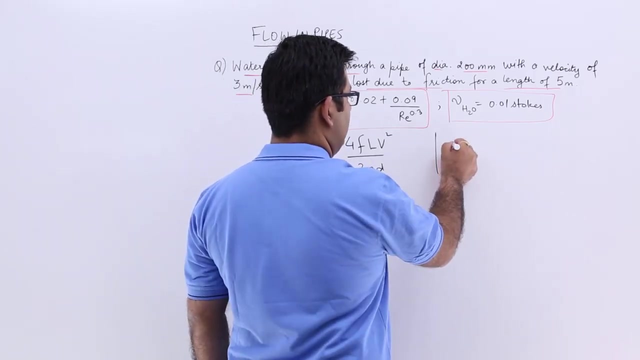 the friction factor is given by this formula and the kinematic viscosity for water is 0.01 stokes. Okay, so it's a very straight forward formula wherein we have to apply the relation, which is: hf is equal to 4 f lb square upon 2 gd. So the dia of the pipe is 200 mm, which. 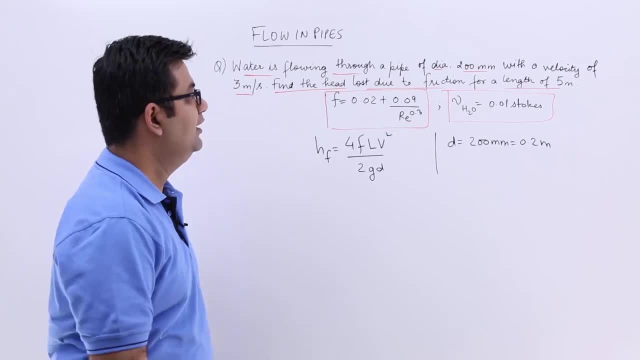 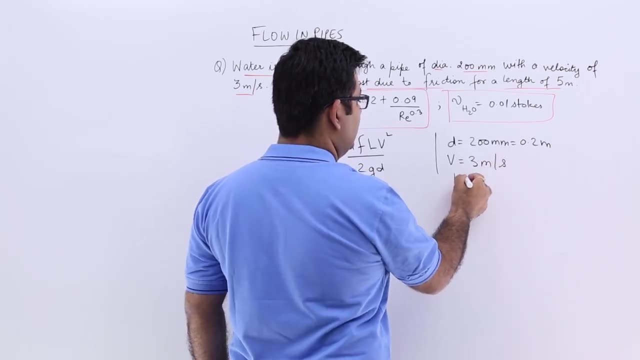 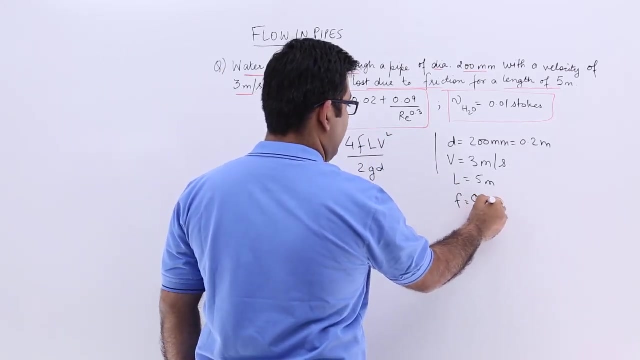 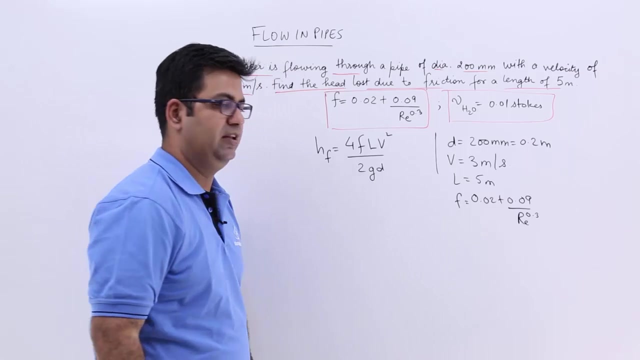 is 0.2 meters. The velocity given to you is 3 meters per second. The length of the pipe is 5 meters. We don't know friction, because it depends on the Reynolds number. So first of all, let's find out the Reynolds number only. So for Reynolds number. 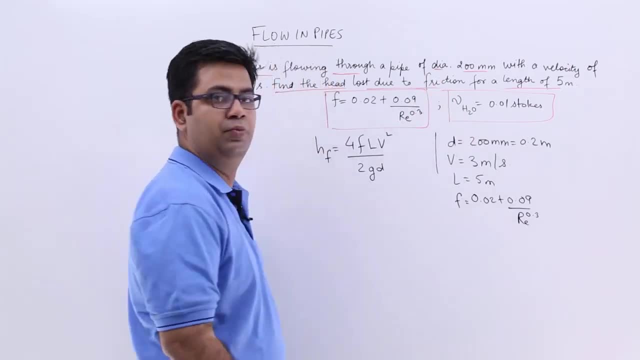 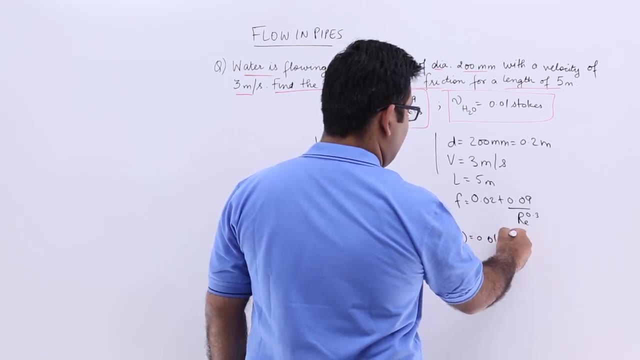 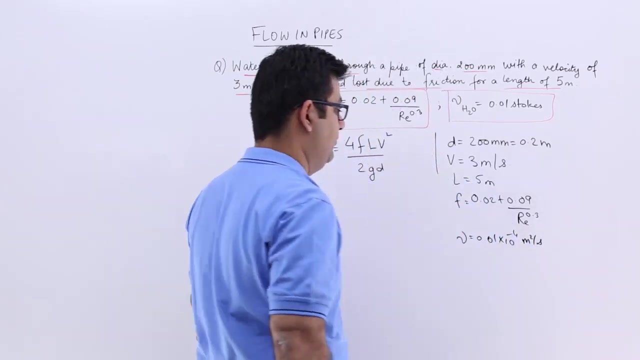 I need v, d and nu. Okay, so what is the value of nu? Nu is given to you as 0.01 stokes. You multiply that by 10 to the power minus 4. You get it in meters square per second. 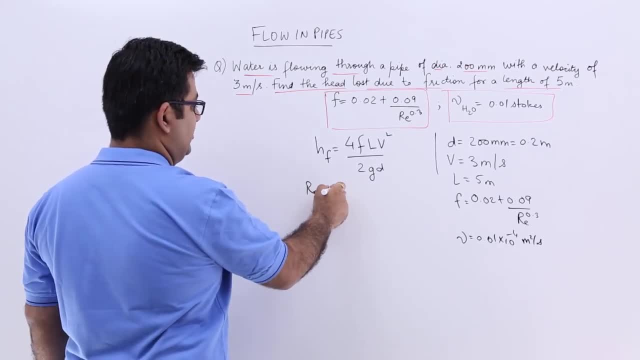 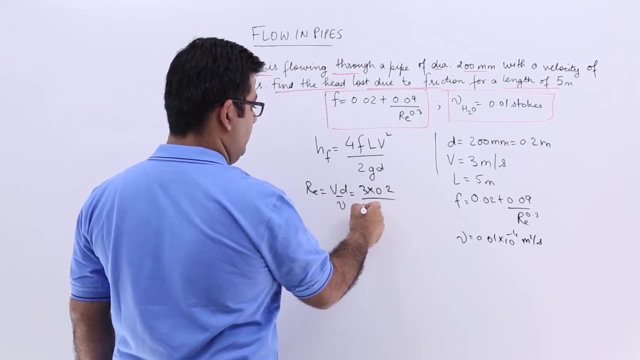 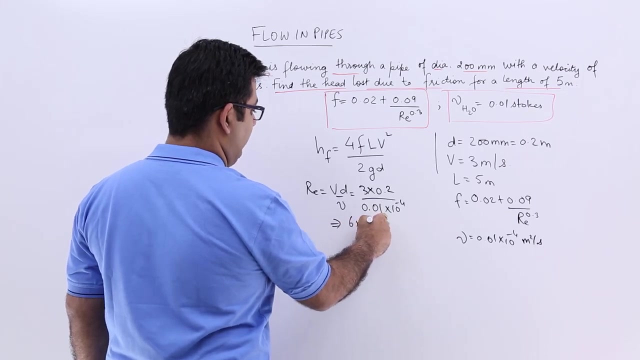 So with this I will be able to find out Reynolds number, which is v d upon nu, that is 3 into 0.2 upon 0.01 into 10 to the power minus 4, and that is 6 into 10 to the power 5, which. 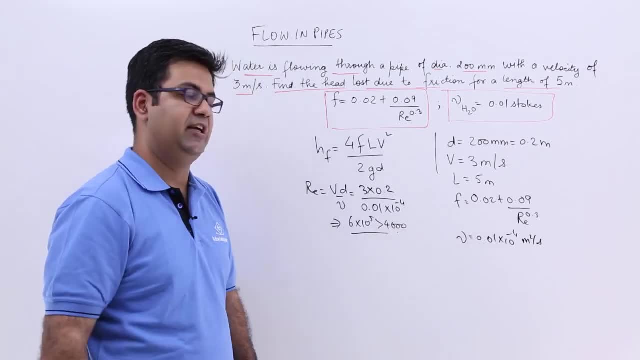 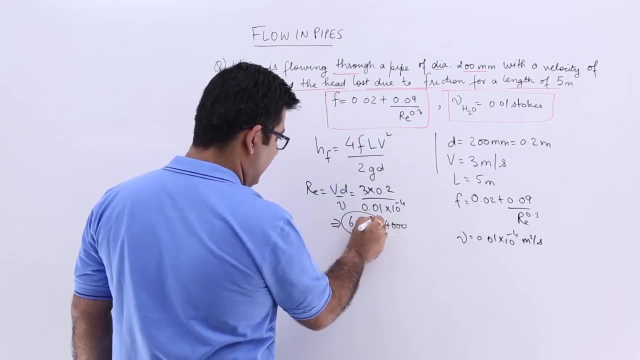 is more than 4000.. Okay, That is. it lies in the turbulent region. Okay, Now, with this value in place, I can put it over here and find the value for the friction factor. So when you put r is equal to 6 into. 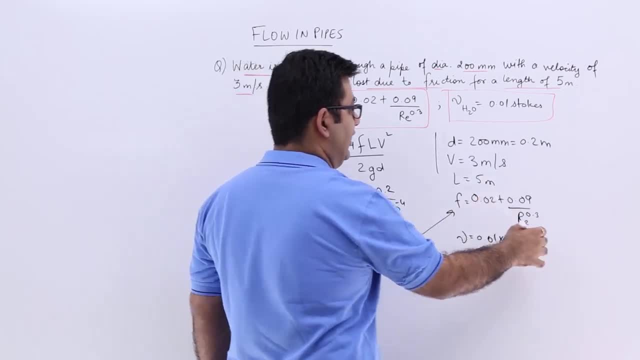 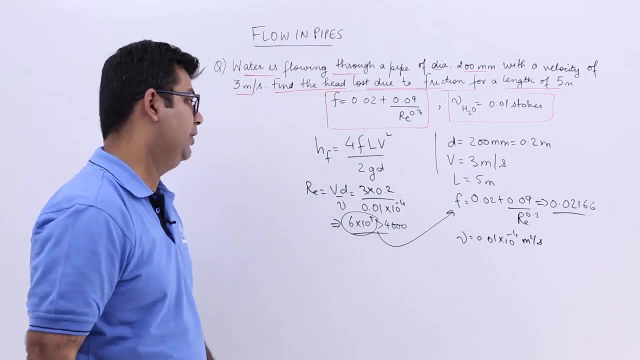 10 to the power 5 over here and you calculate the entire thing, you get a friction factor which is 0.02166.. So this is pretty much that you have to calculate before you calculate the friction head loss. So that will be 0.02166.